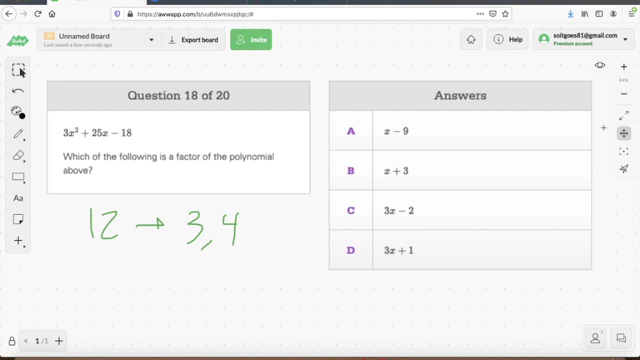 and 12 together to get 12, right. Cause: 1 times 12 is 12.. So another set of factors of 12 is 1 and 12.. So you can say these are all factors of 12,, 3,, 4,, 1 and 12 are factors. 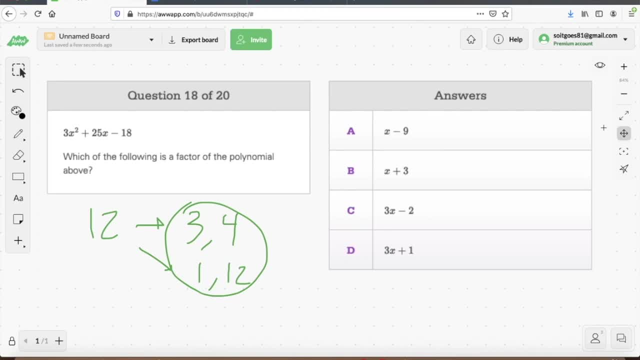 of 12.. Numbers are terms that you multiply together to get 12.. Does that make some sense? Yes, Okay, I mean you do the same thing with like 16.. What are the factors of 16?? Well, obviously, 4 times 4 is 16.. We've got 4 as a factor, But you 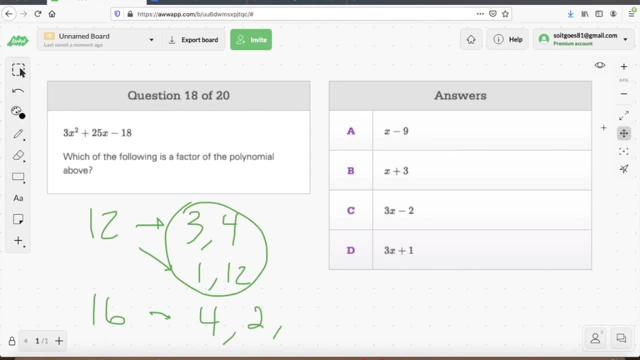 also multiply 2 and 8 to get 16. So another factor would be 2 and 8. And of course 1 times 16 is also 16.. So 1 and 16 are also factors, In no particular order. 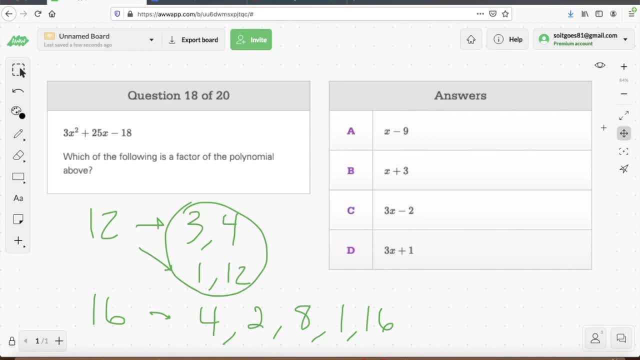 Clearly Right there. But those are all factors, Numbers that you can multiply together to get 16.. Does that make sense? Okay, All right. So there's a way to sort of factor this like algebraically, And it's super annoying, It's super. 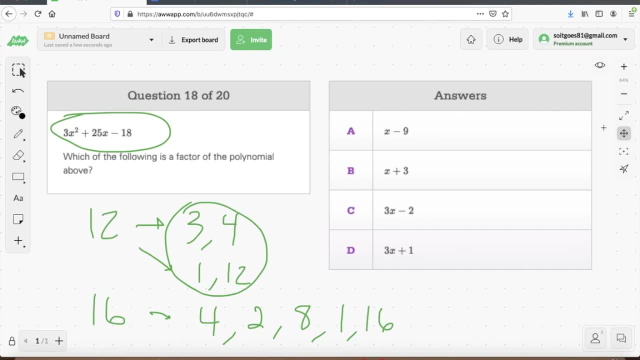 complicated And you don't need to know it for any of the factoring questions I've seen on the Accuplacer, So I'm going to teach you the trick, which is turning it into basically arithmetic with plugging in values. Okay, I'll show. 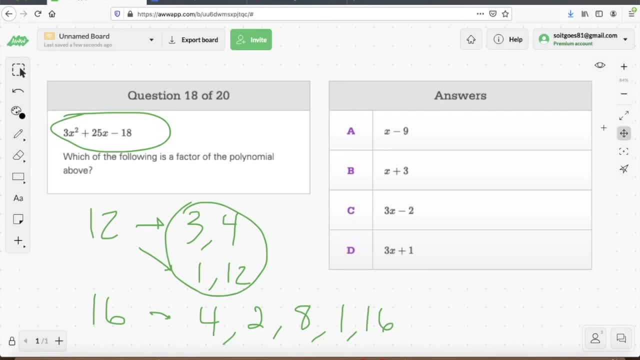 you what that looks like. On all the factoring questions I've seen you can do All right, So I'm going to create a value for X. I have not abandoned the plugging in values strategy Still works, So we're going to create a value for X, X. 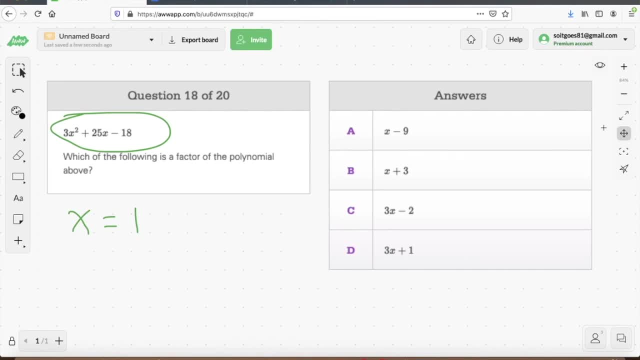 is 1.. 0 might work, I don't know, But we're gonna do. We're gonna start with 1.. All right, All right. So if X is 1, what does this expression in the question equal? Okay Well, 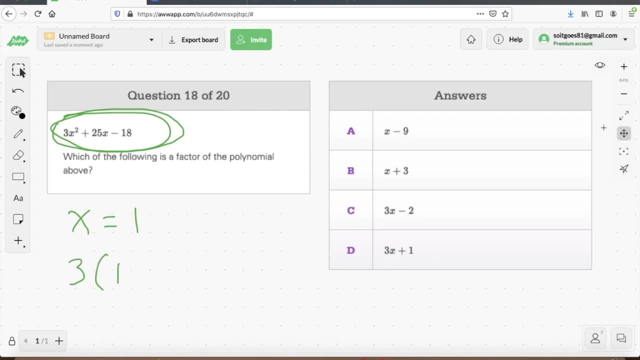 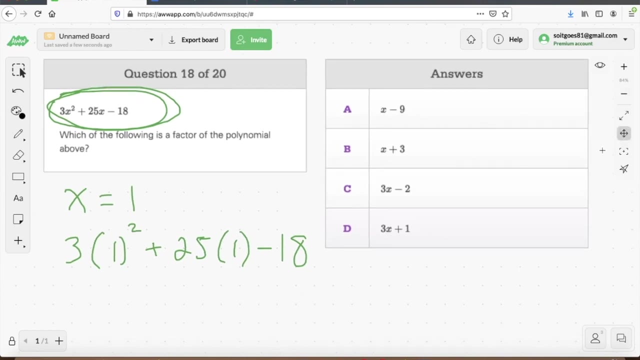 let's just plug in values, So it's 3 times 1 squared plus 25 times 1 minus 18.. Let's simplify this And this will be a good PEMDAS review. Can you talk me through this? How would we simplify this? 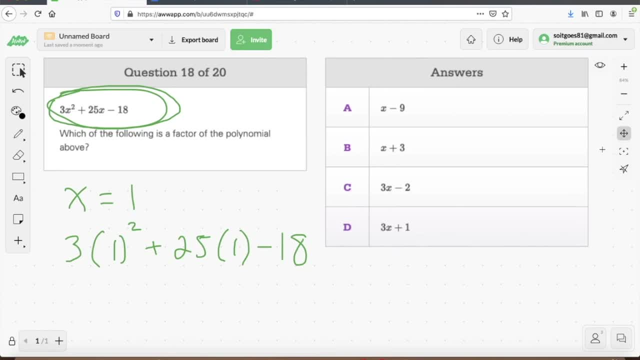 Okay, So What does that equal? I guess You do your exponents first, right Yep Exponents first, Absolutely. Maybe you can work this out. Let me see you simplify this. Okay, So do those exponents first, Absolutely, Absolutely. 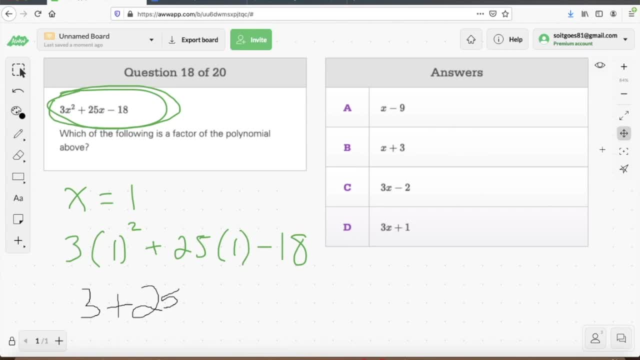 Perfect, I'm gonna stop you real quick. You did this beautifully. I'm so glad you didn't square the 3 here. I'm so glad you didn't right, Because 3 is not being squared, It's just the 1 that's being squared. And what's 1 times 1?? 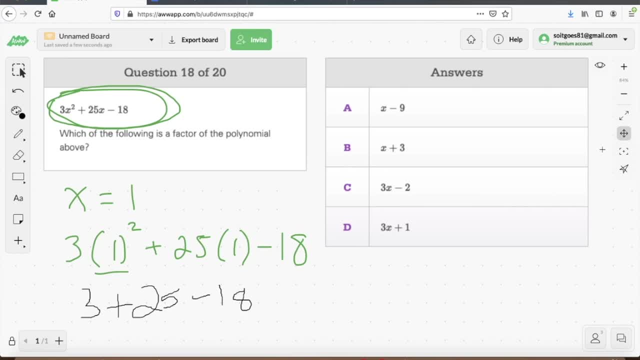 1. Just 1.. So that's 3 times 1, which is just 3.. Beautiful. And of course, 25 times 1 is just 25.. So great job there. I just want to go over that PEMDAS order of operations. there A lot of students want. 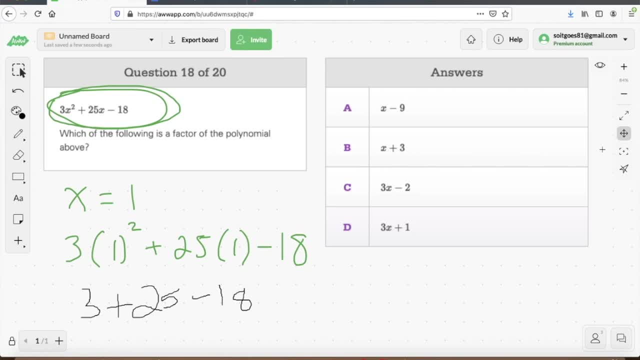 to square that 3.. It's not going to be 9.. It's just going to be 3 on the left-hand side, All right. So what does that give us, by the way, 10. So that's going to get. It's going to be. 3 plus 25 is Yeah, It's 28 minus 18 is. 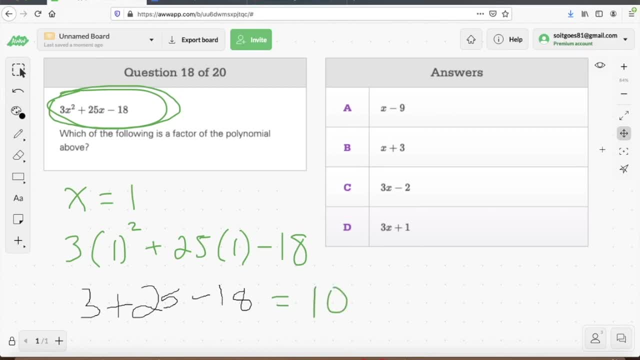 10. Absolutely Okay. So when X is 1,, this expression of the question is 10.. When X is 1.. Okay, Great. Now the question is: which of the following is a factor of that polynome? But when X is 1, that polynomial. 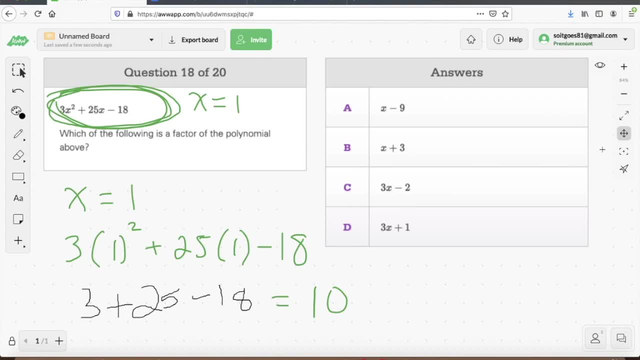 that expression is 10.. So really now we've turned this into an arithmetic question. We're saying: which of the following is a factor of 10?? That's all we're finding now. Which of the following answer choices is a factor of 10?? 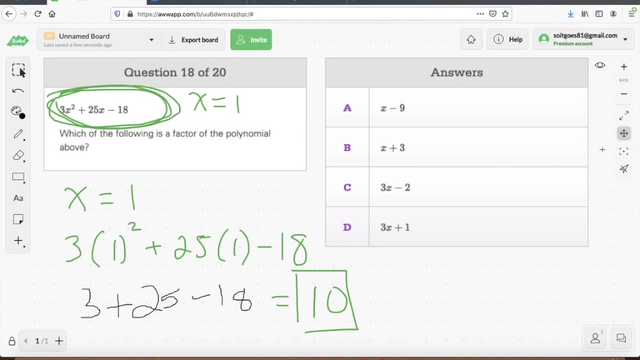 x is 1.. Does that make some sense? Wait, why did you say that again? Yeah, yeah, yeah. So the question is saying which of the following is a factor of that polynomial expression, this big expression up here with the x squared, 3x squared plus 25x minus 18.. All right, But when x is 1, that expression equals 10.. When x is 1.. So we've turned this question now into which of the following is a factor of 10.. Okay, When x is 1.. 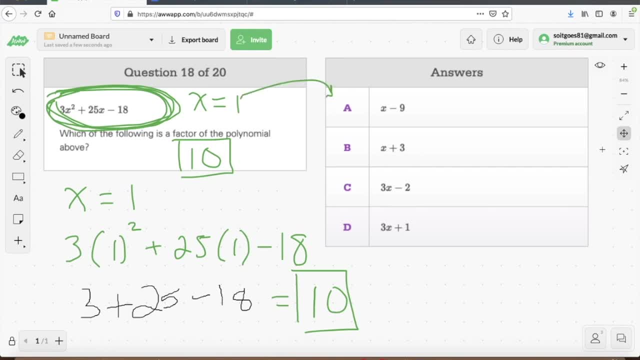 Right, And then we're just going to plug in that 1 for x in the answer choices and see which of those answer choices is a factor of 10.. Okay, It's going to make. that needs to make more sense as we as we do this, as we test these answer choices. So let's plug in a 1 for x in answer choice A. What does that give us When x is 1,? what does that give us for answer choice A? 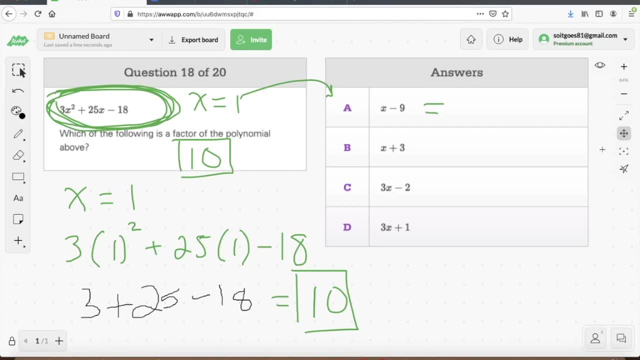 It's going to be a negative Mm-hmm. It's going to be negative for sure. It's 1 minus 9. 8. Negative 8.. Absolutely, That's negative 8.. Okay, Okay, Is negative 8 a factor of 10?? That's to say, can you multiply negative 8 by something to get 10?? 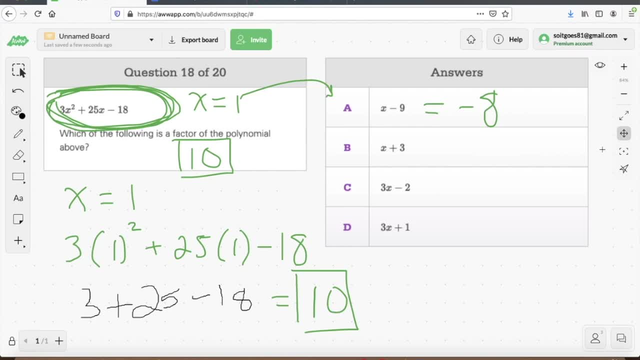 No, No way, No way. So A is gone. Does that make sense? Yes, Beautiful, Let's plug in that x is 1 into answer choice B. Now, that's 1 plus 3.. What's 1 plus 3?? 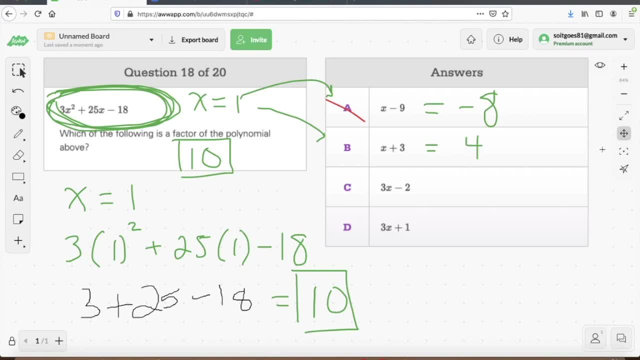 4. 4. Is 4 a factor of 10? No, No, I mean you can't multiply 4 by some whole number at least, And get 10, right, Because 4 times 2 is 8, but that's less than 10.. And then 4 times 3 is 12, and that's bigger than 10.. 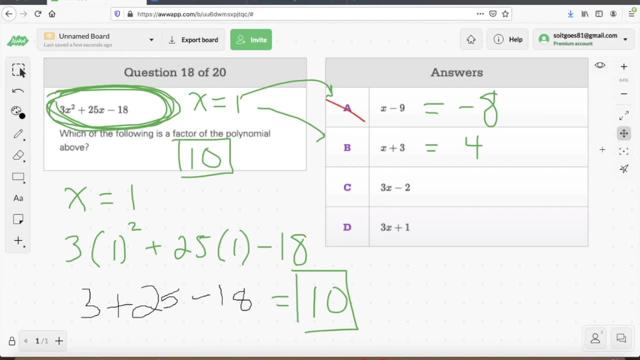 You can't multiply 4 times some whole number and get 10.. So you can also eliminate answer choice B. Make sense? Yes, All right, Let's try answer choice C: That's 1.. That's 1.. Is 1 a factor of 10?? 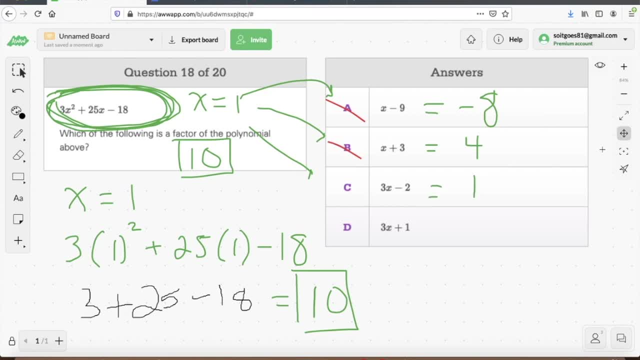 You can do 1 times 10.. You can do 1 times 10?. 1 is a factor of 10.. That's true, So we'll keep answer choice C. What about answer choice D? No, that's 4.. 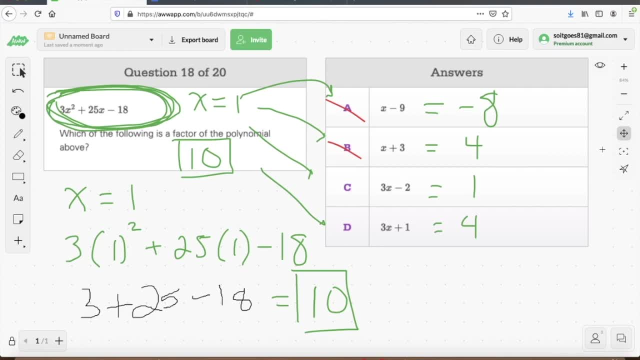 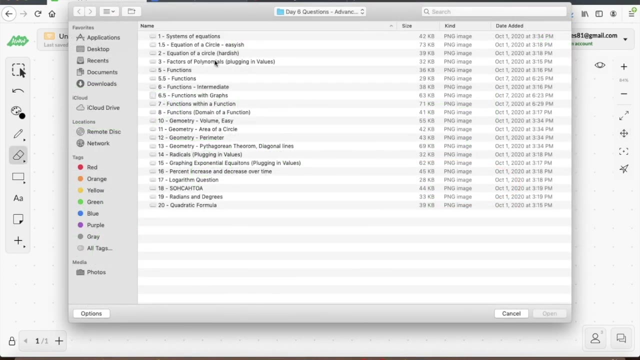 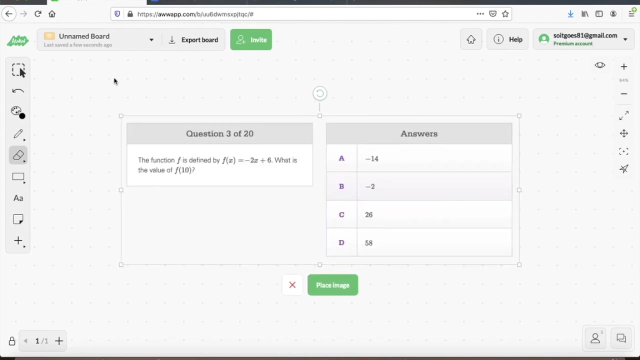 That's 4.. Is 4 a factor of 10?? Is 4 a factor of 10?? Oh no, No way. Yeah, Answer: choice C: All right. So basically what I'm doing here, we're just going like concept by concept in the sort of advanced algebra and functions section of the Accuplacer. 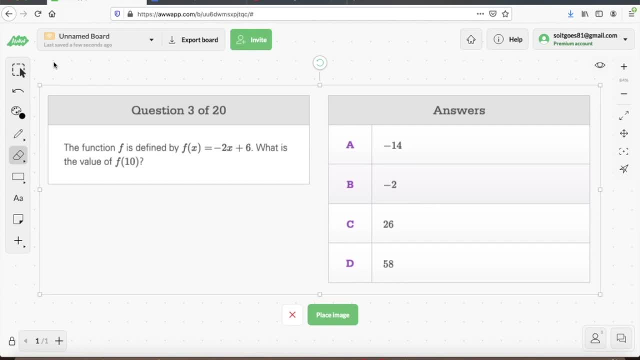 That's all we're doing here. There's just some real specific concepts like factoring, like the equation of circle, and functions, which we've talked about a little bit, I believe, on day 4.. Day 4, part 2.. 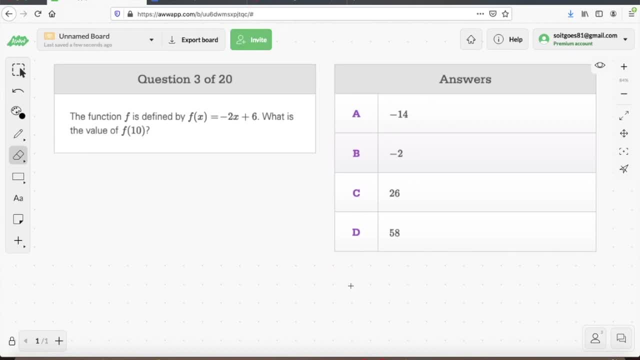 We talked about functions a little bit, a little bit, but I want to get back to them, Okay, Because you're definitely gonna see some functions questions on the Accuplacer And I want to really have this down. So I want to spend some more time on functions right now. 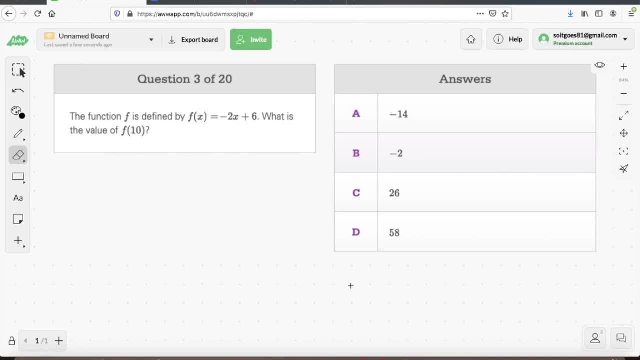 Go ahead and read this question for me. We'll talk about functions in general and I'll show you exactly how to solve this. The function f is defined by f of x equals. Did I write f of x Perfect? F of x Perfect, Yeah. 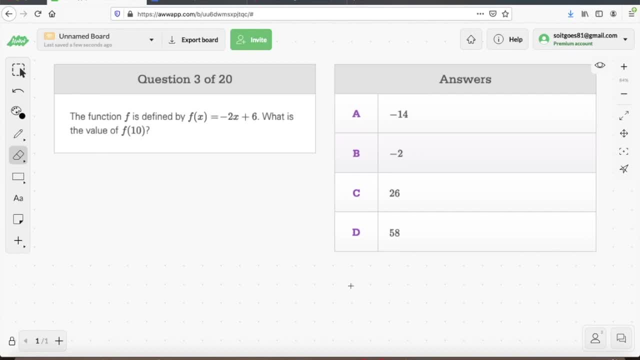 Equals negative 2x plus 6.. What is the value of f times 10?? So that's actually read f of 10, right, Just like up here is f of x, Oh, f of 10.. Yeah, yeah, yeah. No, I mean, and I get like a lot of students think you're multiplying f times 10.. That's not true. No, I mean, and I get like a lot of students think you're multiplying f times 10.. That's not true. No, I mean, and I get like a lot of students think you're multiplying f times 10.. That's not true. 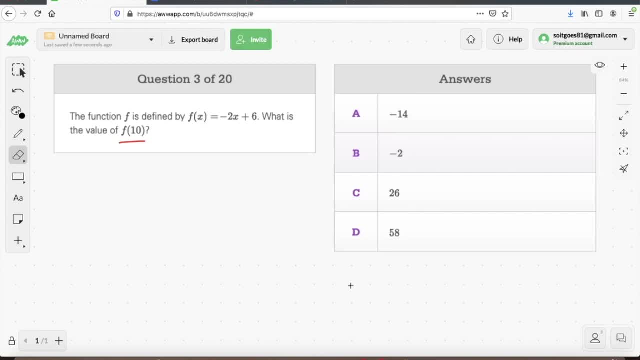 That's not what it means. This is function notation. Okay, and we're gonna review that here in just a moment. Okay, and we're gonna review that here in just a moment, I think. previously I gave you an example of a real simple function. I'm gonna do the same thing here. 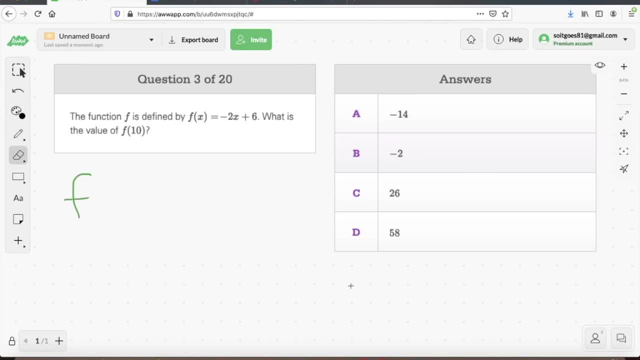 This is worth reviewing. Okay, This is worth reviewing. If we had a function like this: f of x equals 3x plus 1.. Okay, There's a function And um And function notation throws a little bit of weight on that. 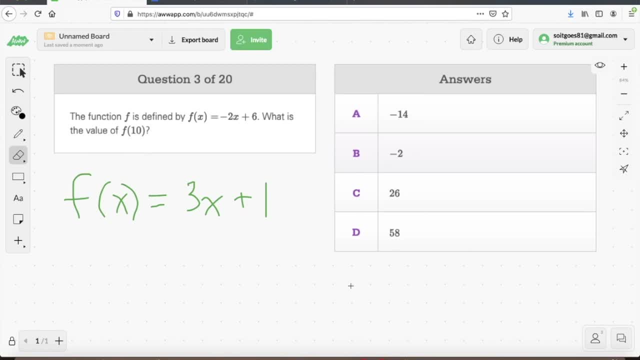 I don't know what to do with that. Okay, don't even worry about that. It's basically the same, as you know. it's the same as the equation y equals 3x plus 1.. It would graph the exact same way on the xy axis. 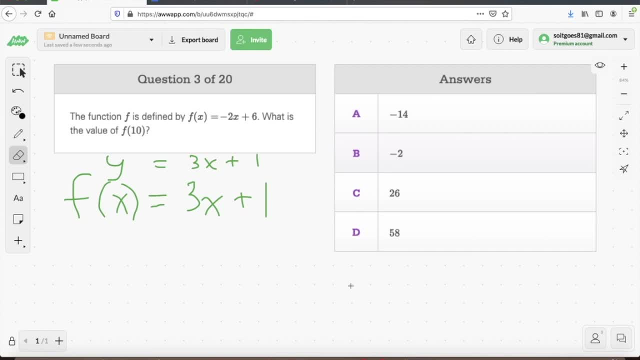 In fact f and y are interchangeable. Sometimes I just describe f as fancy, y Okay. So it's really, it's the same concept, just a different way of writing it out. But I'll show you why. function notation is actually kind of handy. 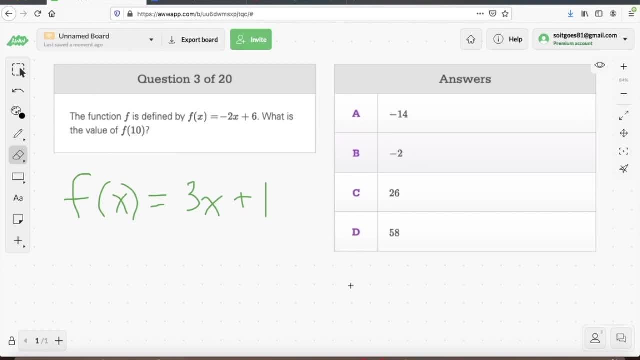 Okay If I said okay, if I said find Okay. Okay, Find f of 2.. Okay, Find f of 2.. All that means is where there was an x, now there's a 2 in the function. 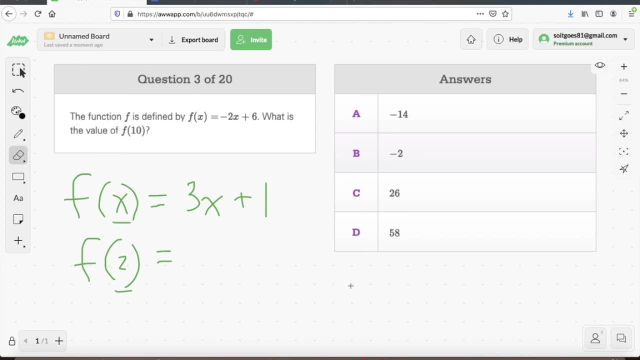 So you're replacing all the x's with 2's. That's it, Okay. So what's f of 2?? It's just going to be 3, not times x, but times 2.. That's 1.. Does that make sense? 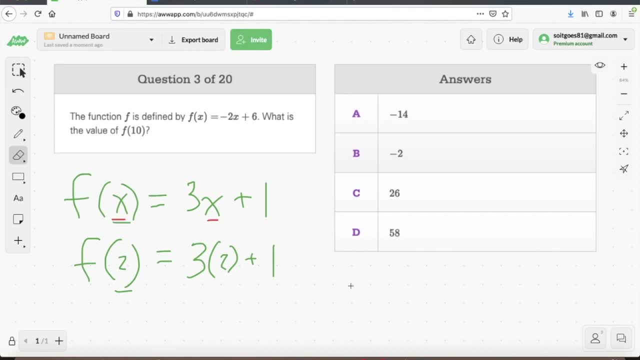 Yes, Literally all you've done is you've taken where there was an x, you've replaced it with a 2.. A question like this is really a breeze. once you understand the concept of a function, what function notation means? So I could say: f of 2 equals. 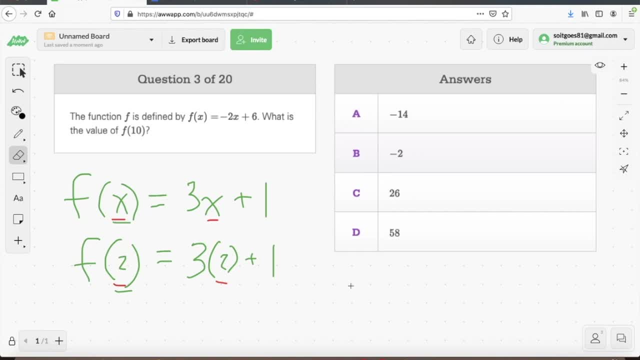 I'm just going to simplify this: 3 times 2 is 6, plus 1 is 7.. So f of 2 is 7.. Does that make sense, Right? Yes, Okay, So when your input, and this is how I recommend thinking of functions. 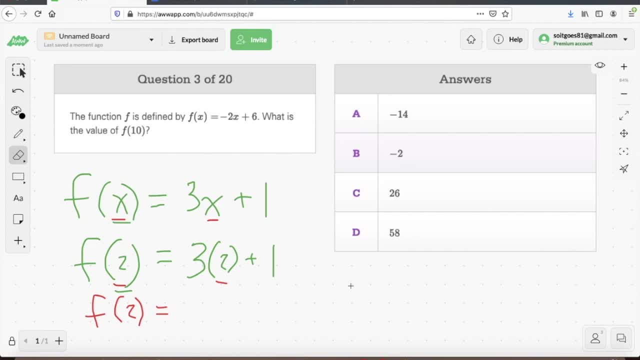 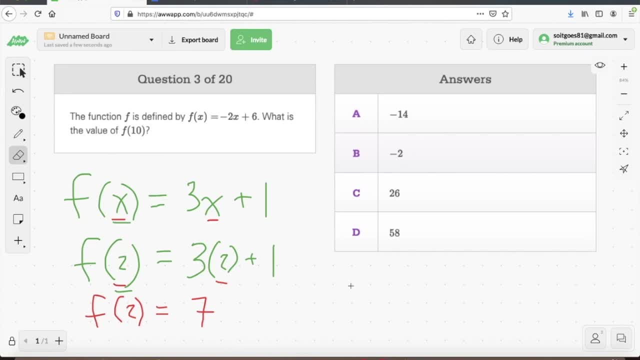 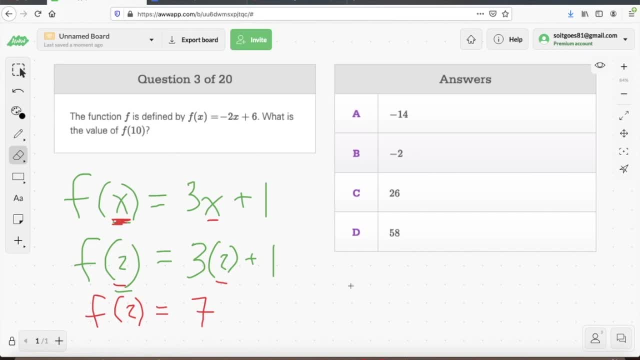 plus 1 is 7.. Okay, So when your function has 2 things about it, x is your input. so when 2 is your input in the function, your output is 7.. Inputs and outputs: X is your input. 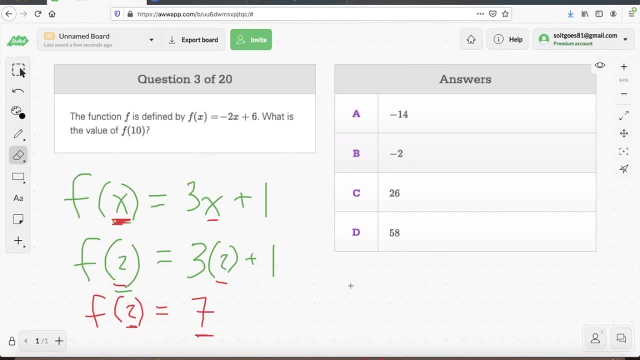 F of x is your output, Or f of 2, or f of 3 or f of 4 is your output? For whatever that input, x is Okay. Let's do it again. okay. So it's, you know you're probably going to see a number of function questions. 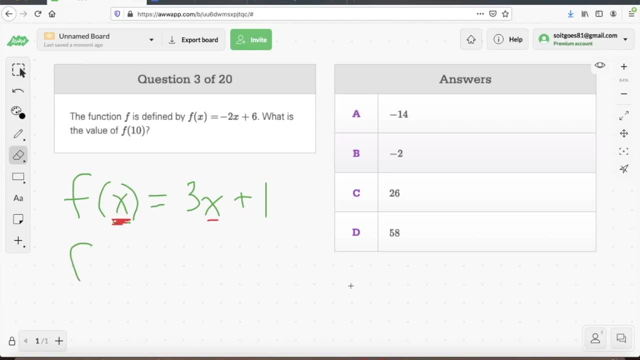 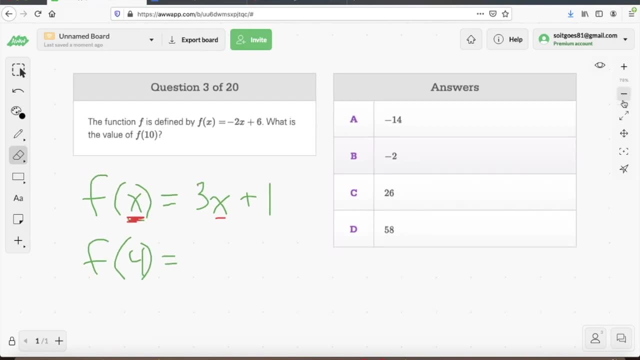 I just want to really get this down. Let's find f of 4.. What's f of 4?? In fact, I want to see you work this out. Can you show me what is f of 4?? Okay, So I'm going to work that out on the whiteboard. 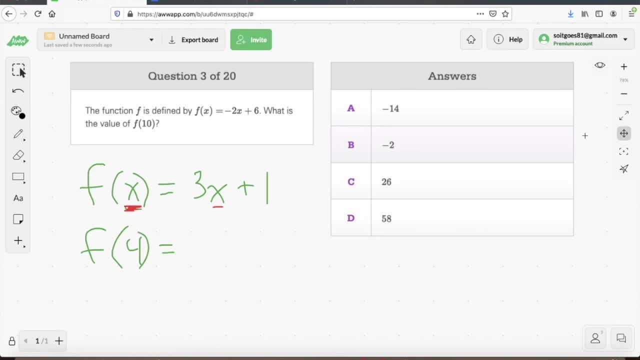 Do you want me to write the 4?? Yeah, I just want to see, I want to see Plug it in: Looking good, looking good, Great Okay. So I'm going to start with f of 4.. Okay, 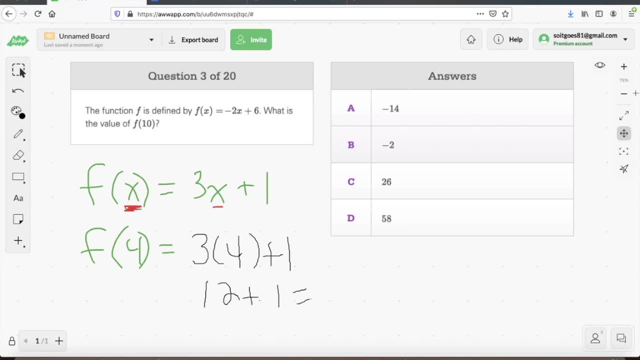 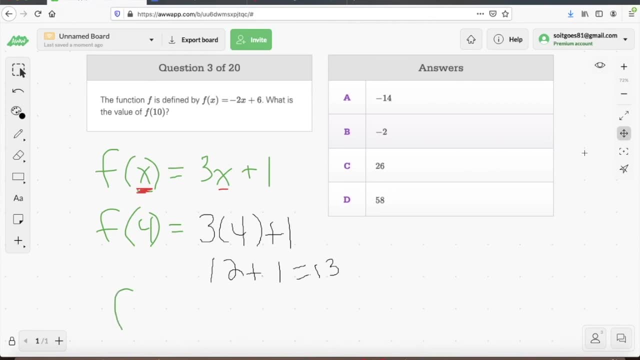 Great, Excellent. So you would say. you would say: f of 4 equals 13.. Exactly, Exactly, That's it, That's it. Another way to express that is basically like when your x value is 4, your f of x value. 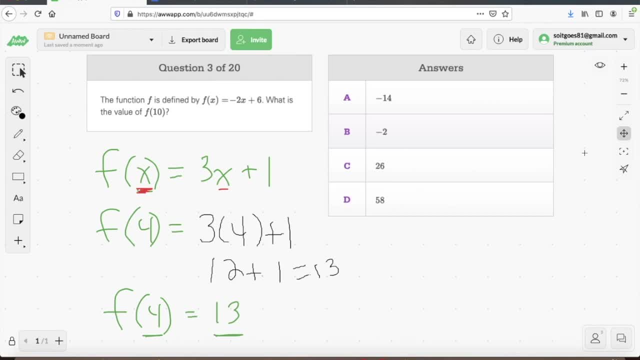 or your y value is 13.. Okay, Your f of x value or your y value, same thing. F of x is just fancy y, So you could graph that the same. you know that point on the xy axis. That would be the point for comma 13 on the xy axis. 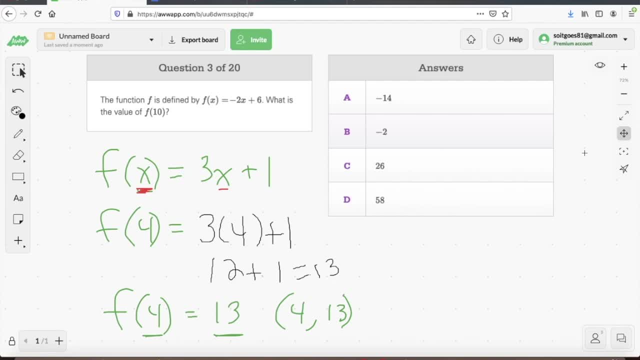 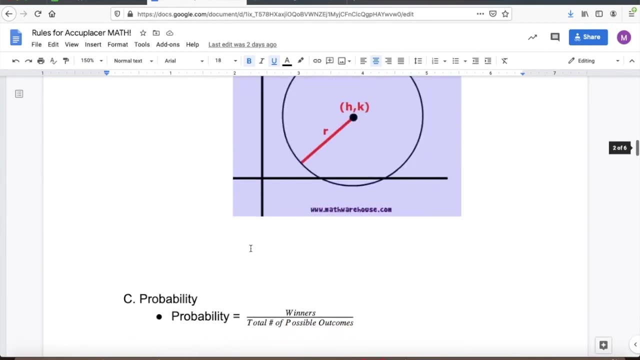 Okay, Okay, And I've got that on the rules for Accuplacer Math real quick. I do want to go over functions again Somewhere here. Where are my functions? There we go, There we go. Basic concept f. 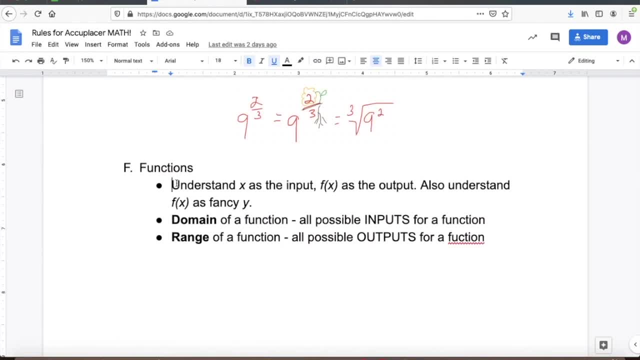 This part right here: Understand x. This part right here: Understand: x is the input, f of x is the output, And then understand f of x is fancy y, especially if they give you a graphing question with functions. Whatever your f of x value is, just make that your y value. 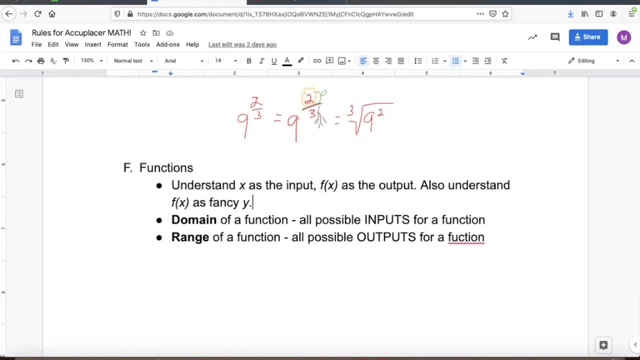 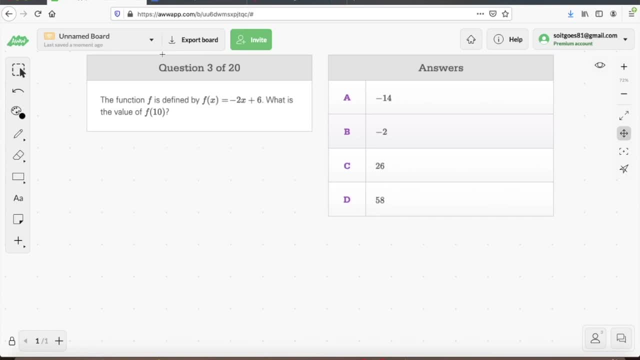 It's the same thing, Okay, And we'll practice that. All right. So let's go back to the question ahead. I just want to review what functions are and how they work. Just understand them in terms of inputs and outputs. 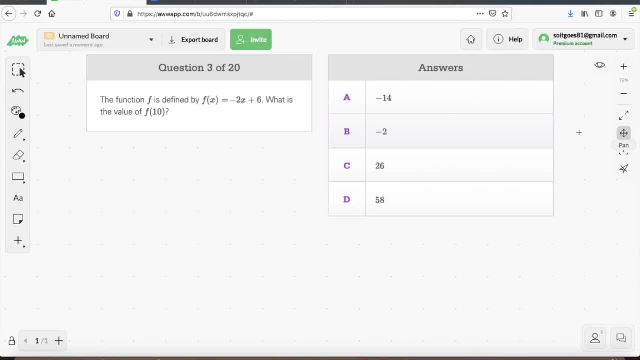 Read the question again one more time for me, because I think this question is actually really really easy. if you understand what functions mean, Go to read the question please. The function f is the y by f of x. equals negative 2x plus 6.. 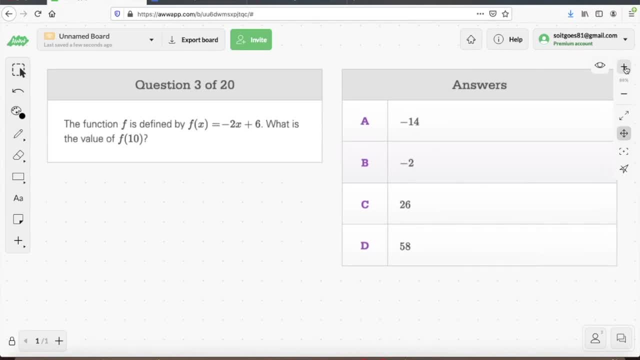 What is the value of f of a? I can't even do it. F of 10.. You got it. F of 10.. You got it. You got it. All right, You know how to do this. Where there was an x in the function, now there's a 10.. 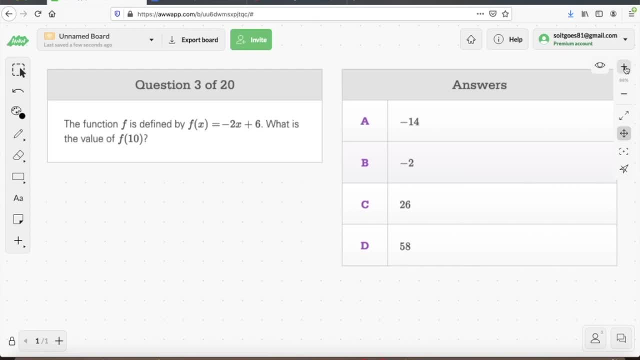 Let me see you plug it in. That's all it means. That's all it means. Okay, So I'm going to go ahead and do the next one. I'm going to go ahead and do the next one. Okay, So I'm going to go ahead and do the next one. 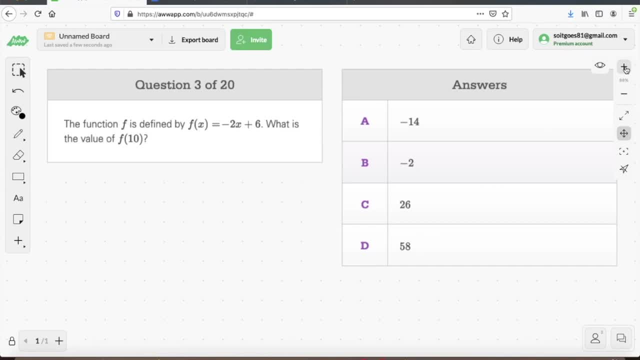 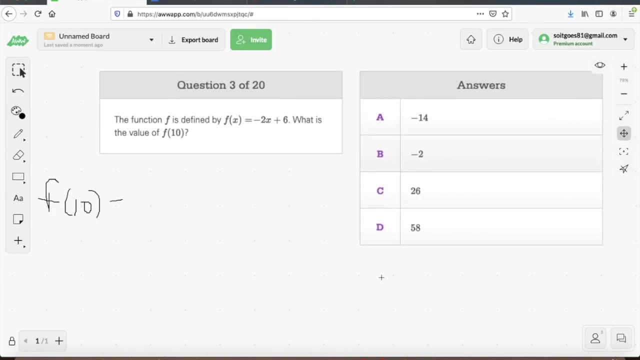 Okay, So I'm going to go ahead and do the next one. Okay, So I'm going to go ahead and do the next one. That's all. it means Absolutely Looking good, looking good. So, All right, Let's simplify it. It's just PEMDAS here, right? We don't need. well, there's. 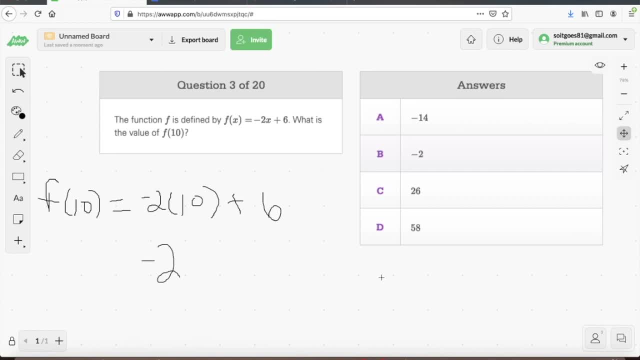 nothing calculated in parentheses, no exponents. Do that multiplication? Beautiful, Beautiful, Come on. What's the right answer here? A Answer choice, A Bingo? Oh, I just raised it. There we go. Beautiful, Easy, if you know. 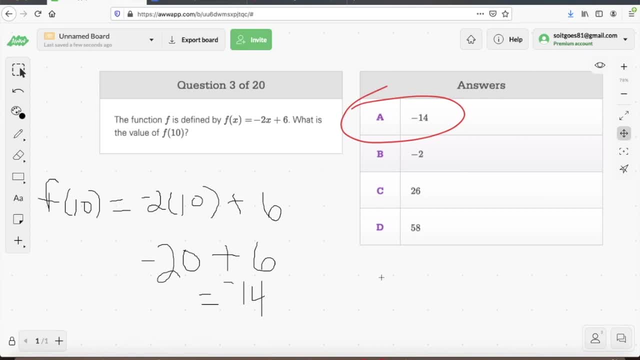 what function notation means. Yes, Does that make sense? Yes, Don't be intimidated by it, Just find it. whatever is you know in the parentheses, that's your input. So 10 is your input for X. Really, it's a plugging in values question. 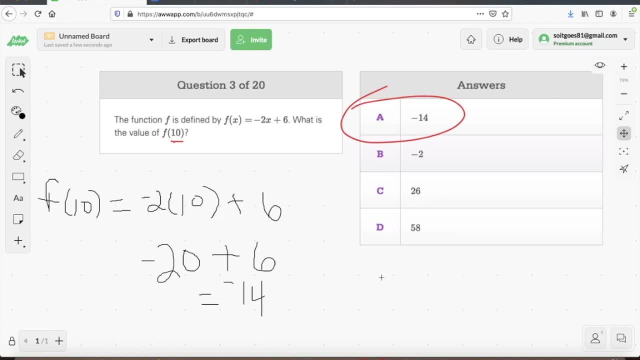 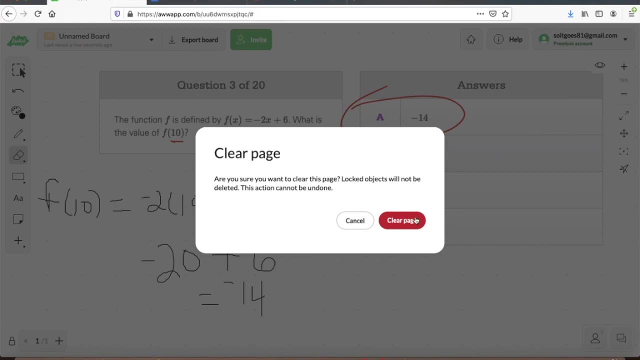 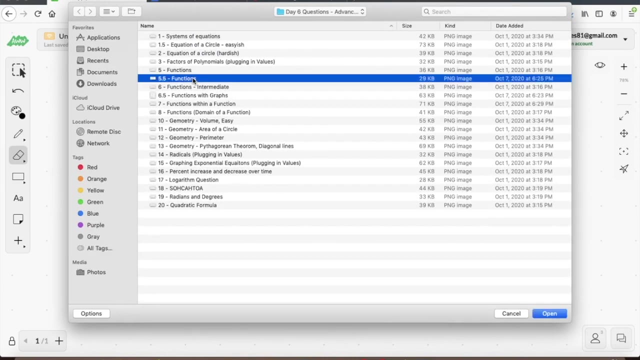 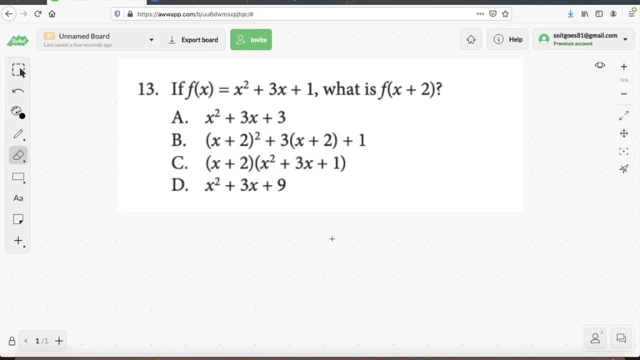 disguised as a function question. You're just plugging in 10 for X, Okay, Okay, All right, Let's do some more functions, All right, I like this one. This one's funny. It looks really scary. It's really scary. It's not. Go ahead and read this one for me, please. 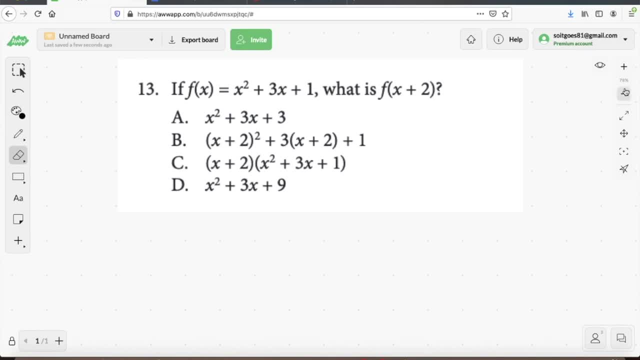 F of X equals X to the second, plus 3X plus 1.. What is? How do you say that? I have to say F of X plus 2.. Okay, F of X plus 2.. Remember in the last question, right where we were finding F of 10?? Remember that, And 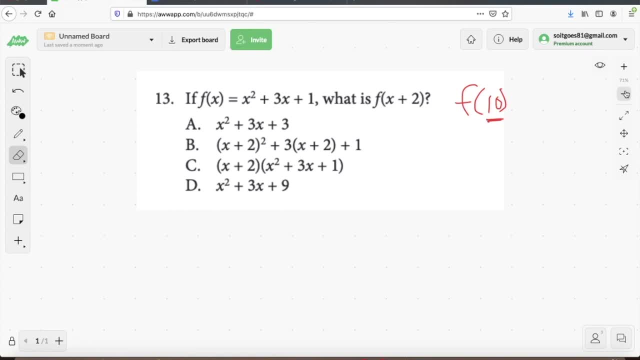 I said: whatever is in parentheses, that's your input for X. Okay, Same thing here. What's your input for X? What's your input? It's a thing in parentheses: X plus 2.. X plus 2 is your input, Absolutely. So where there was an X, now there's just an X plus. 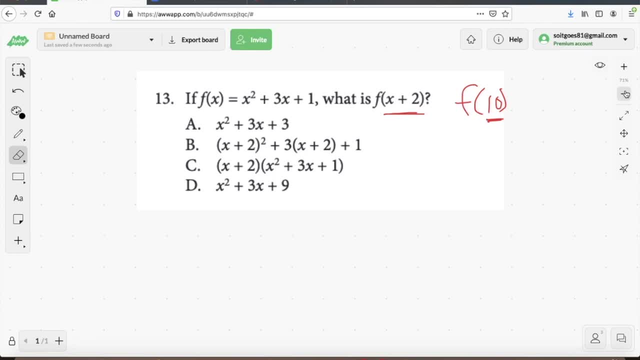 2. So plug it in. Plug in X plus 2 in place of X into this function, right here. Does that make sense? Yes, All right, Let me see you do that. Looking good, Looking good, Looking great Okay. 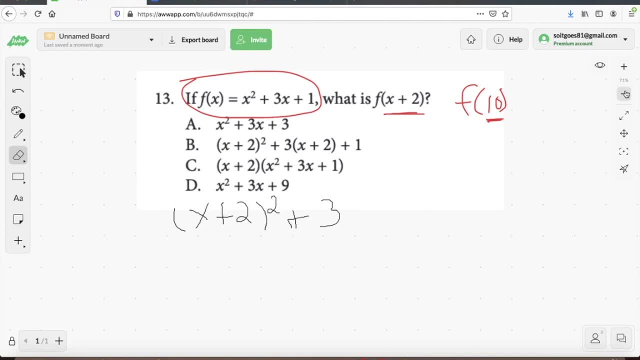 Okay, where there was a nexus, now there's X plus two- Magnificent, All right. I'm going to stop you real quick, because the temptation is to multiply all that out like FOIL. that X plus two squared. distribute that three times X plus two. It's very tempting. 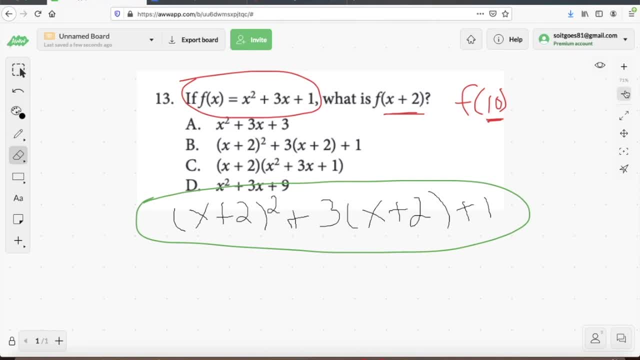 to do that, But I want you to look at the answer choices real quick, Keija, Tell me what the right answer is right now. B Answer choice B. It's exactly what you have here. All they're testing you on is if you. 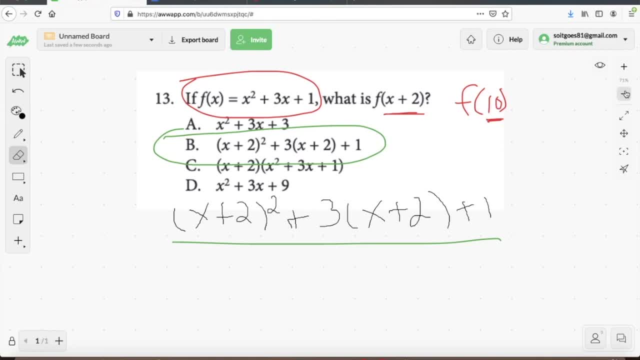 have that. concepts of inputs and outputs straight. That's all. That's all. Where there was an X, there's now X plus two. That's it. Any questions about that? No, sir, All right. All right. Inputs and outputs. Just keep your inputs and your outputs straight. 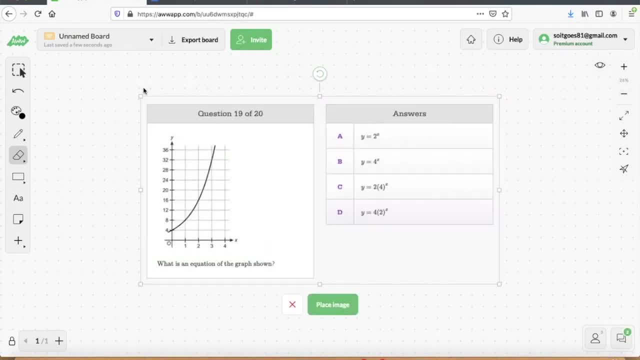 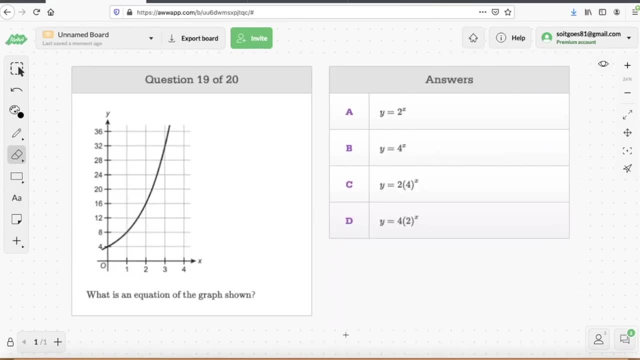 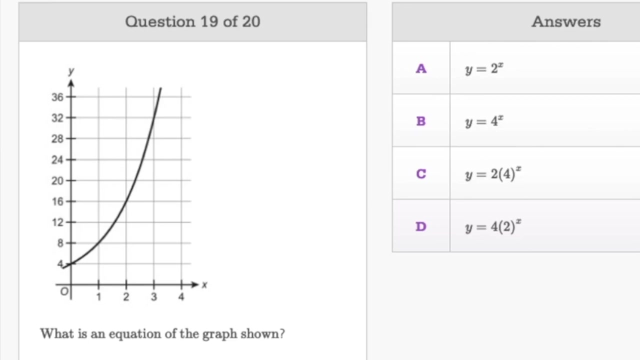 and you're good. These look like scary questions, This one here especially. It's very scary, But it's not bad. Go ahead and read this question for me, please. What is an equation of the graph shown? Okay, Okay, Now, this is a funky curve here. Okay, Funky curve. This is a graph of an exponential. 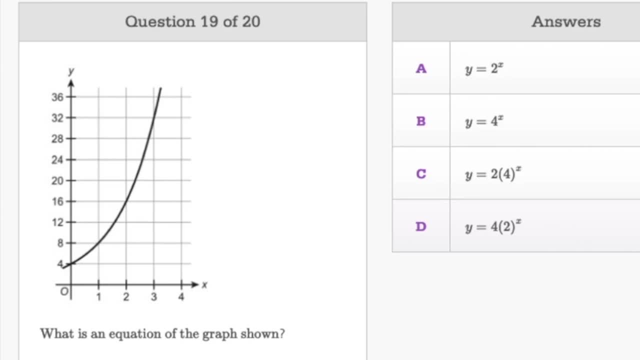 equation. Okay, You get funky curves up, for we're talking about exponential increase, or a funky curve down. We're talking about exponential increase or a funky curve down. We're talking about exponential decrease. Okay, And notice in the answer choices, by the way, all of the answer choices. 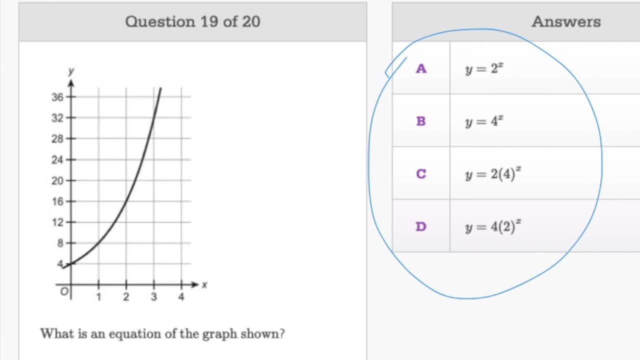 have X raised to a certain power, Or sorry, all the values are raised to the power of X. I should say That's why it's called exponential or exponential growth. It's because X is an exponent here. Okay, Okay, Now just looking at the answer choices, I don't know which. I don't know how to graph. 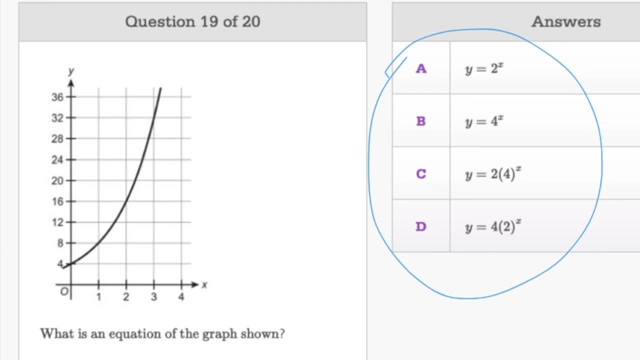 any of those, Right, Okay, Right, It's sort of like in the way you can just sort of like use, you know, slope and the Y intercept to do: Y equals MX plus B. It doesn't work like that with you know, there's no. 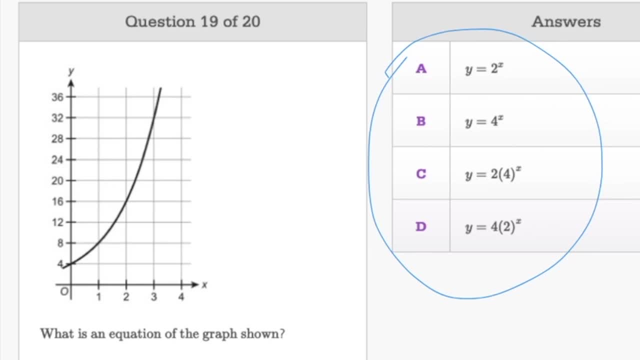 trick to that, like that with exponential equations. But let's look at this graph again. Let's look at this graph right here. Anytime they give you a graph, they're giving you a bunch of X and Y values that you can always test. 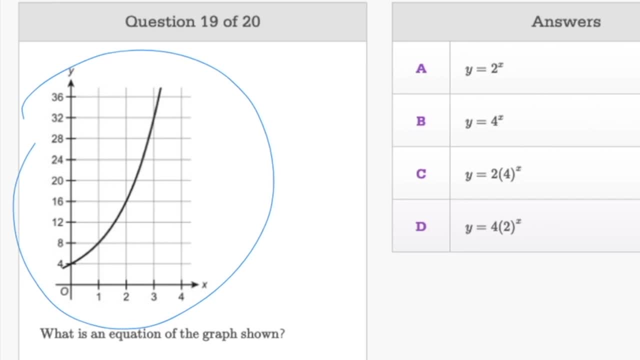 A bunch of X and Y values. Okay, A bunch of X and Y values. For example, I know, when X is zero for this equation in the graph, when X is zero, what does my Y value have to be Zero, No, 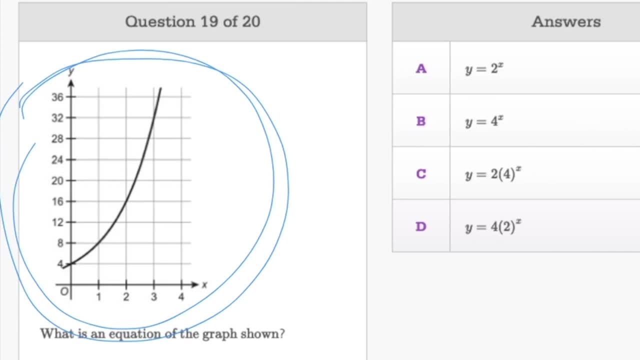 No, When X is zero, what does my Y value have to be in the graph? In the graph Four? It's four, Absolutely Right. It's that point, right there, Right. Zero comma four. Does that make sense? 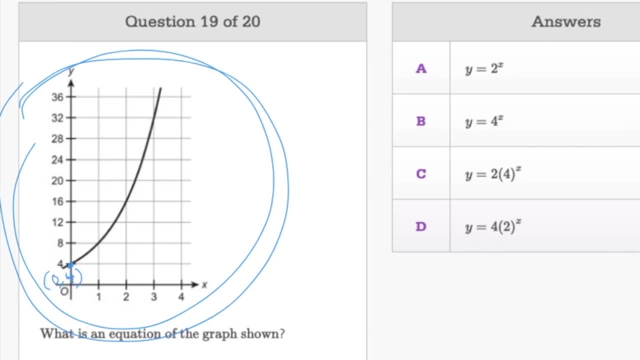 Yes, Okay, I know, when X is one, what's my Y value have to be Eight. Oh, Eight, Eight, Absolutely Right. That's the point, right there, That's the point. One comma eight. So when X is one, Y has to be eight. 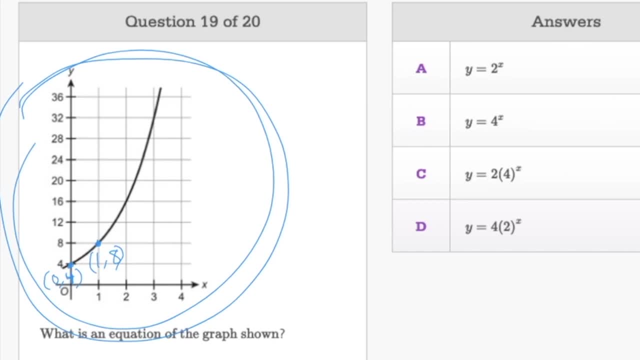 When X is two, what's my Y value? have to be Sixteen, Sixteen. That's the point, right there. Two comma sixteen. Okay, Two comma sixteen, Does that make sense? Why I say: you've got like a bunch of X and Y values you can sort of test. 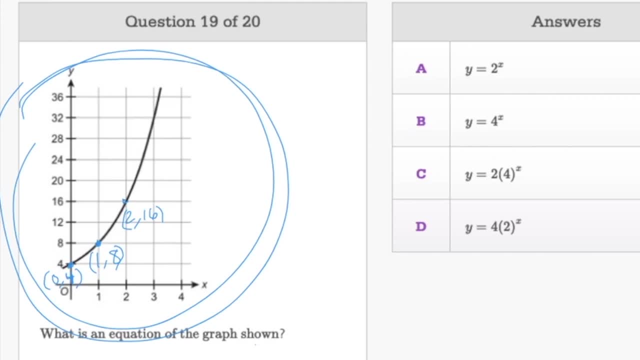 Yes, Okay. So all we've got to do now is take those pairs- and I don't know how many it's going to take here- but plug those into the answer choices, and the right answer has to give us a true statement for all those. 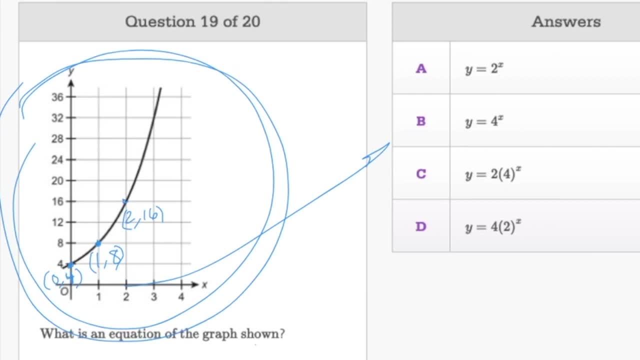 We've got more. if we need to, We can plug in three and thirty-two if we need to. Okay, Let's start. Go ahead. What's up? No, I'm going to try. I'm going to solve it. 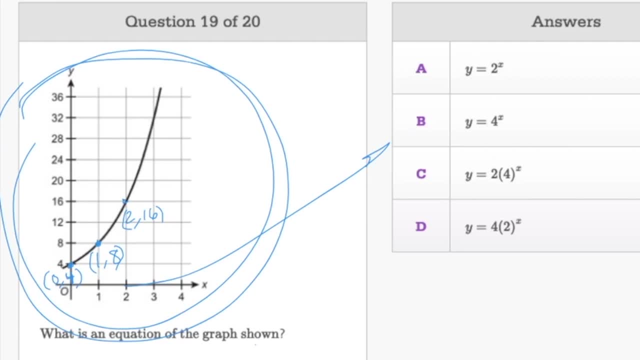 It'll probably answer my question. Okay, Okay, Let's start with. Let's do this, I'm going to. Let's start with one and eight. Okay, Because you know what things to the power of one are right, What's? 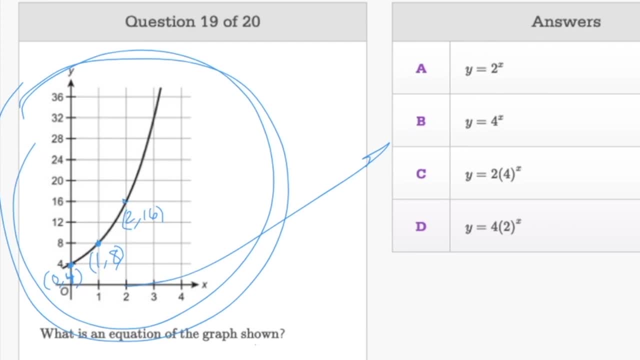 Like, for example: what's two to the power of one? Two to the power of one? one, Uh-huh. What's two to the power of one? One? No, No, Oh two, It's just two, right. 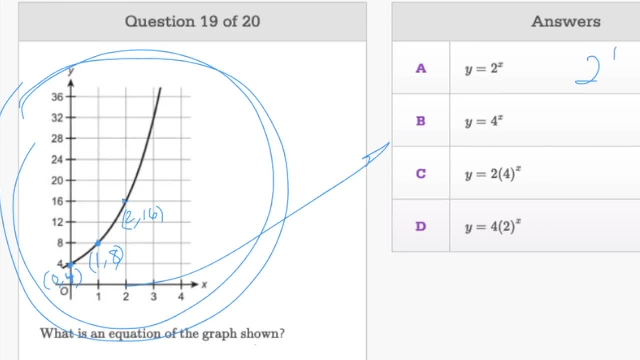 Yeah, It means two one time. basically, Two to the power of two is four. Two to the power of three is eight. Two to the power of three is four. Two to the power of three is eight. Right, Is that familiar? 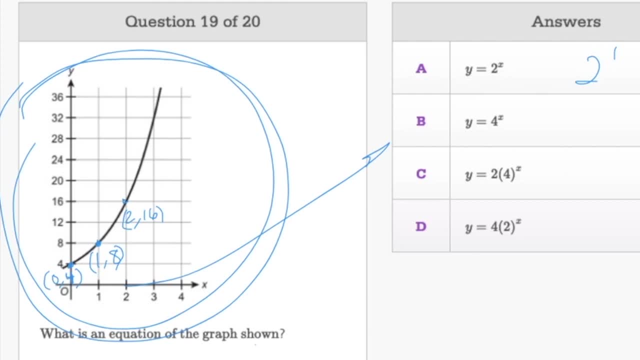 Kind of how those exponents work. Yeah, Okay, The reason why I was tempted to plug in this zero and four pair right here and we could do that. I mean it would totally work, but students get tripped up on things to the power of zero. 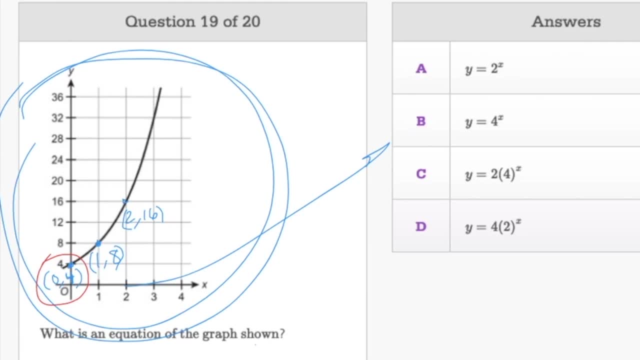 Things to the power of zero throws everybody off. Well, we might come back to it, I might address that here in just a minute. But things to the power of one, anything to the power of one, is itself Right. So two to the power of one is going to be two. 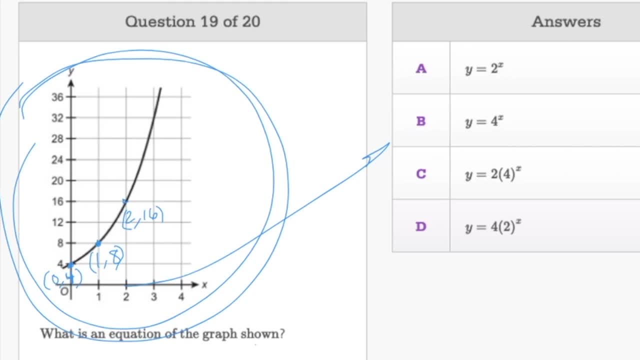 Four to the power of one is going to be zero, Three to the power of three is going to be four, Eight to the power of one is eight, et cetera. Okay, All right. So let's do this. Let's plug in our X and Y values into answer choice A and let's see if we get a true statement. 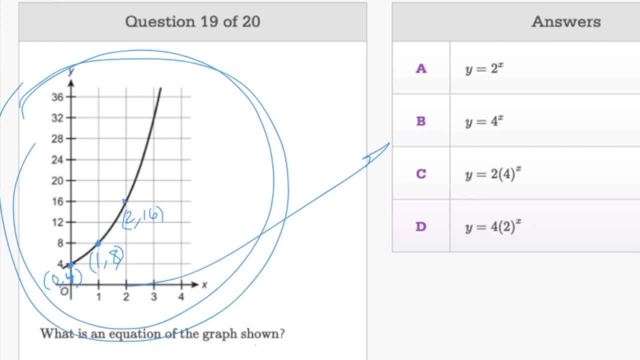 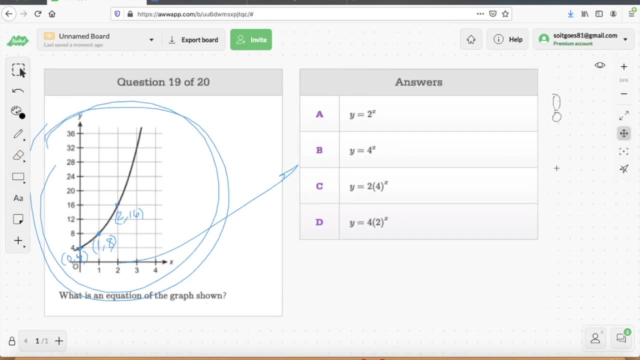 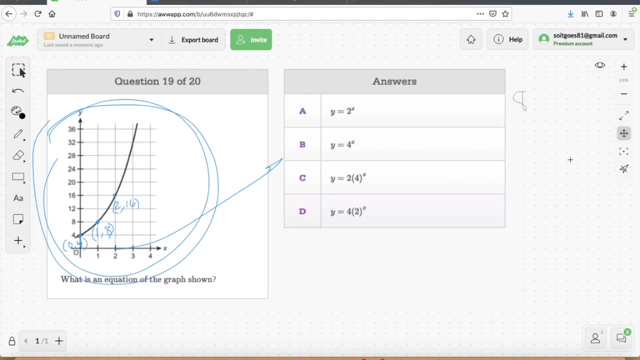 Okay, So we're plugging in a one for X and an eight for Y. Can I see you work that out on the whiteboard? Well, it looks like eight. You're good, I can tell It looks close to an eight. 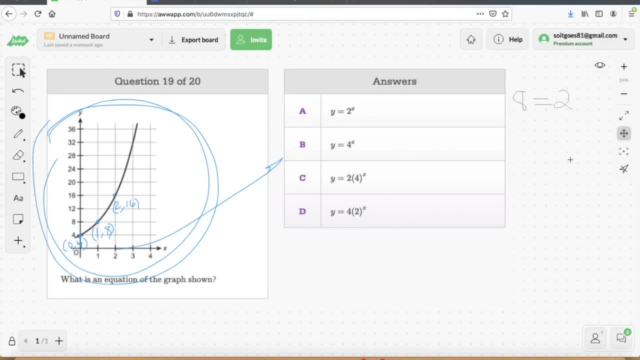 Okay, Oh, I see what you're saying. Uh-huh, All right, You're right. Two to the power of one is just two. So is that a true statement? No, No, And we know the right answer. has to give us a true statement, because we know when X is. 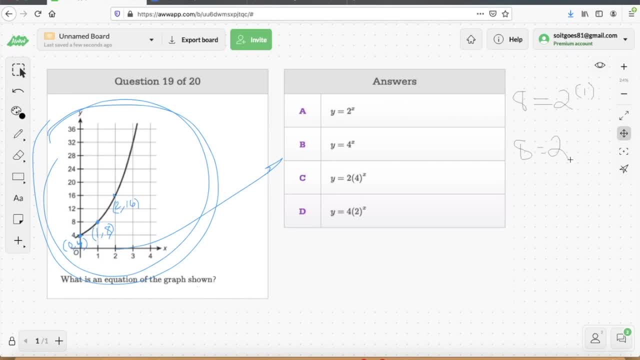 one Y has to be eight. It's on the graph. So answer choice A: Okay, So answer choice A is gone. Make sense? Yes, Great, Let's do the same thing for answer choice B. Let me see you plug in that one and eight. 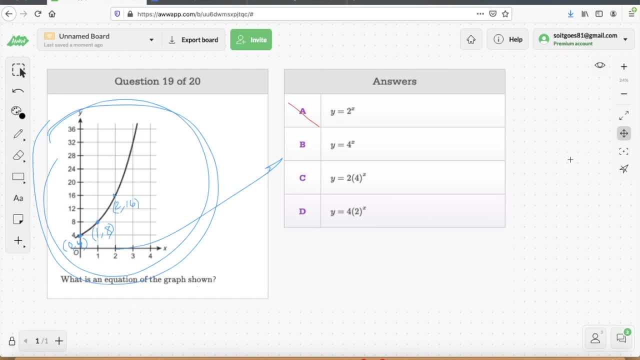 once again, that's not true. that's not true. 8 does not equal 4. last I checked, so answer choice B is gone. this is not bad, is it? 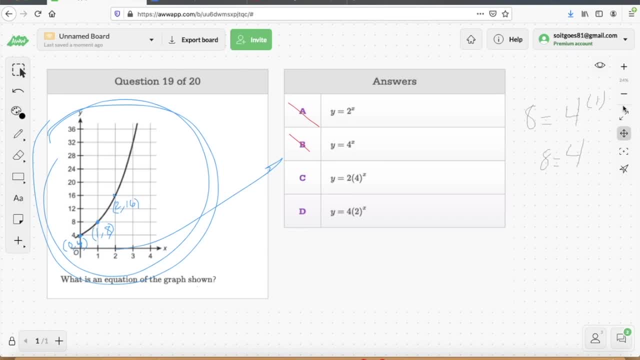 no, no, once you realize again, anytime they give you a graph, they're just giving you a bunch of x- y values to test. works for parabolas, heck. works for lines. clearly works for this funky curve here. this exponential equation works for anything on the x- y axis. 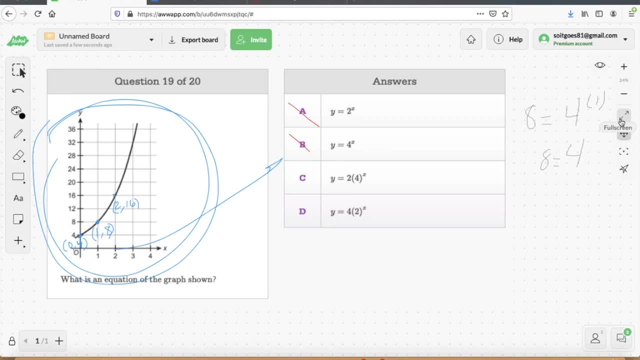 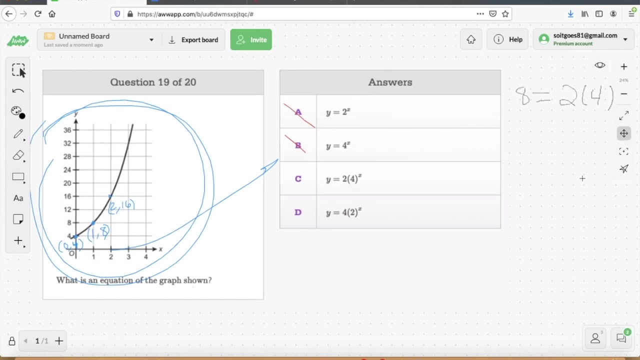 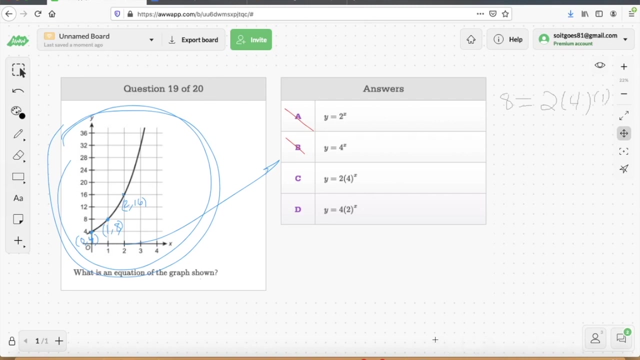 circles. for that matter, it works alright. answer choice C: let's try that. I'll clear some space, oops. alright, yeah, 8 equals 8. that looks good. let's keep C and we'll try. answer choice D: I'm not going to lie, D's looking pretty good too. 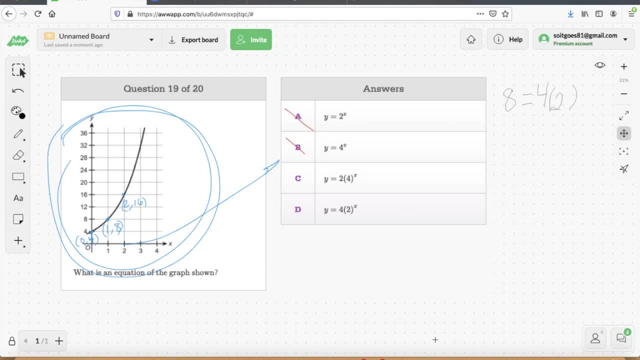 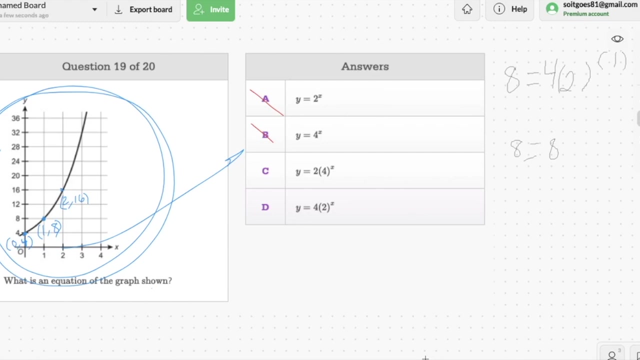 8. so C and D both work. ok, you tell me right now, Kiesha, you tell me what do we do now? it is either C or D. you know, it is a different value. it is a different value. it is a different value. yeah, absolutely, let's plug in a 2 for x. 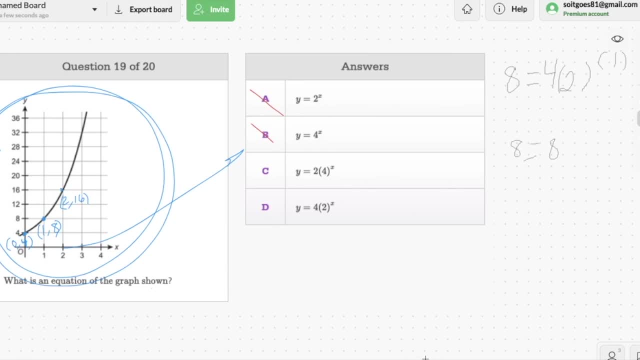 and a 16 for y. let's do that again. if you're really comfortable with 0 as an exponent, you can plug in 0 and 4. that would be totally cool. we're going to do that here at the end, but start with 2 and 16. 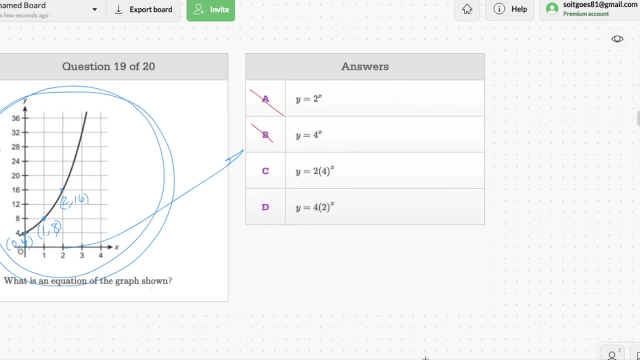 and we're just plugging in A and B are already gone, so we don't have to worry about A and B, so we're just plugging them into C and D. do you know how to increase the way? increase the width of your, of your pencil? 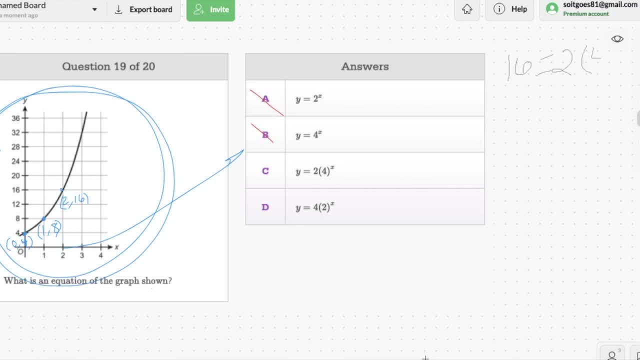 on the whiteboard. do you know how to do that? I just want to make sure this is showing up for everybody I can see. I just know anybody working on a phone might have a little trouble seeing those lines. you want to increase the width a little bit. 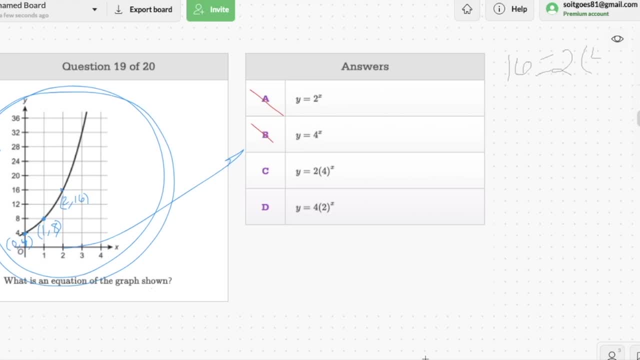 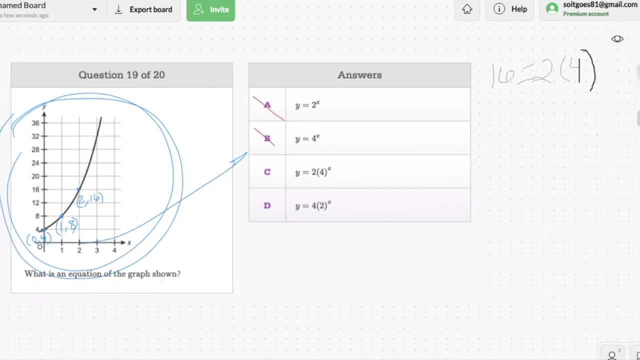 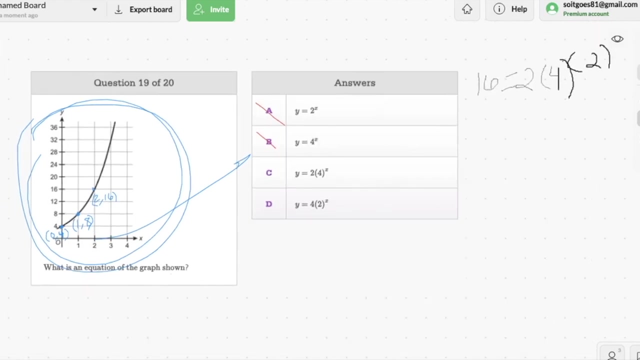 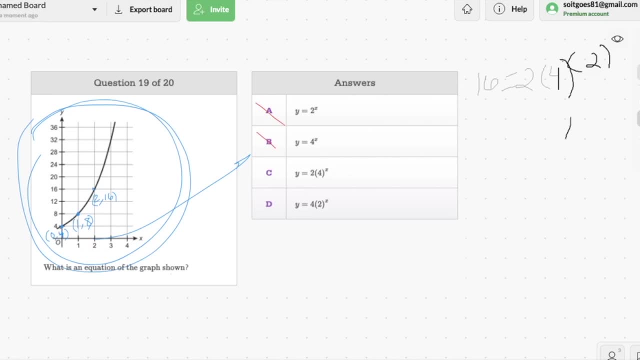 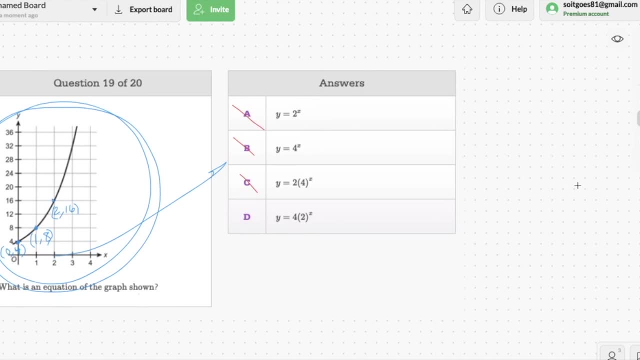 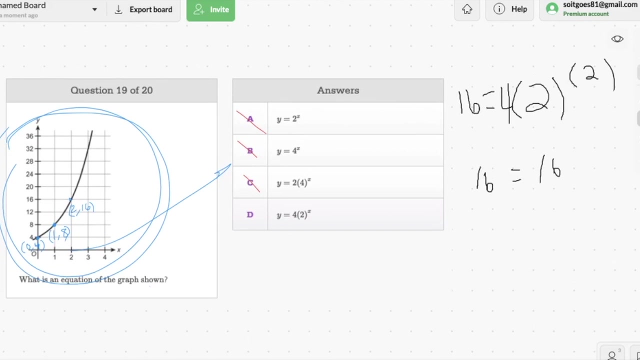 You're good. Yeah right, Absolutely right, Because 2 squared here is 4.. Times 4 is 16.. Absolutely, So you get 16 on the right-hand side, 16 still on the left-hand side. Answer choice D: 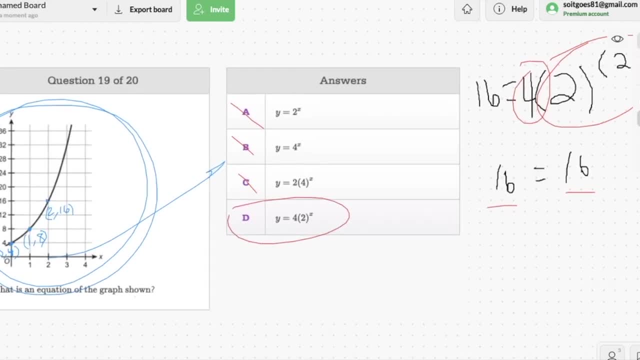 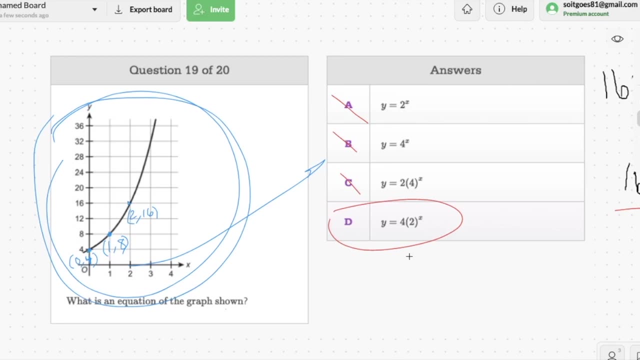 Bingo. Any questions about that? No, Okay, All right. I mean it looks like they're testing you on exponential equations, which kind of they are, But again, you can use that plug-in value strategy which is so freaking handy. 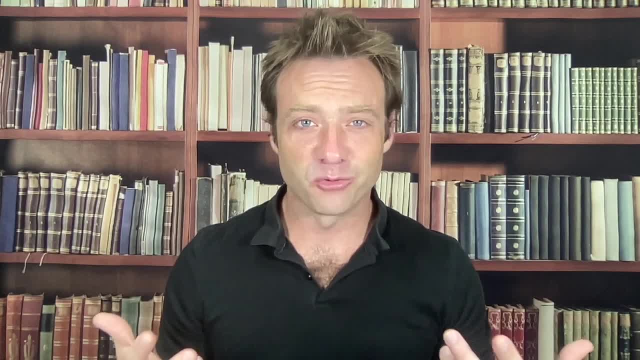 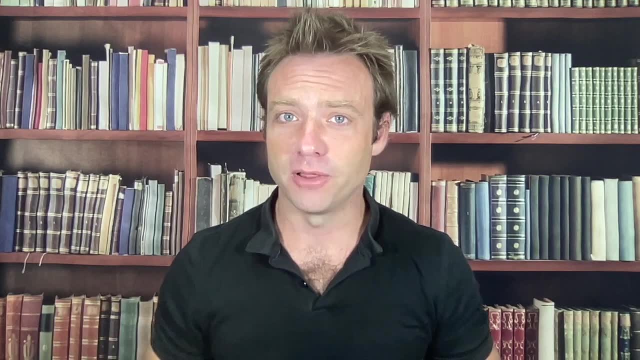 So handy. I hope you guys enjoyed those answer explanations from the advanced algebra and function section of the test. Now don't forget: if you like this video and you're serious about passing the Accuplacer math test, then you definitely want to access the full version of Accuplacer math crash.